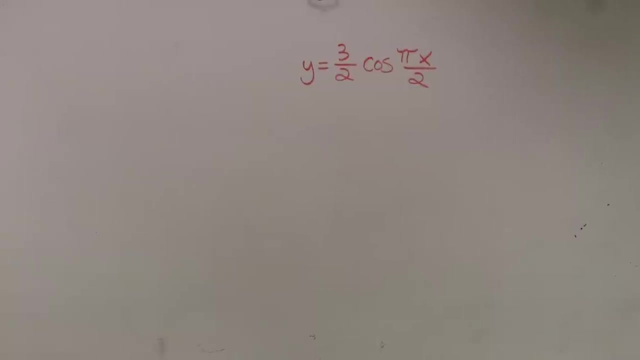 So if we have the equation, y equals 3 apps times cosine pi, x over 2, what we want to do is we want to find the amplitude and the period for these two equations. So there's a couple of simple rules for our amplitude and period. So the amplitude, if you guys remember, is: 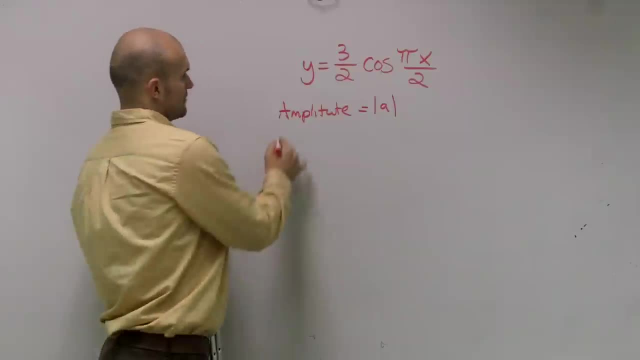 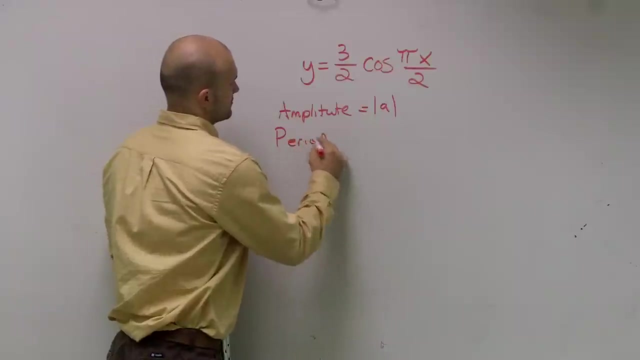 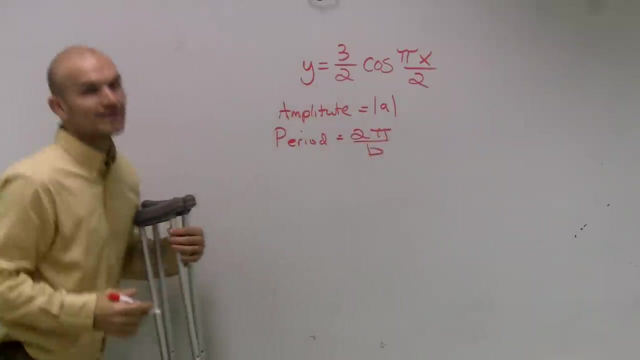 just going to be the absolute value of a and the period is going to be equal to 2 pi over b. Now, in case you guys have not written it down to you, you can write it down. You want to remember. where am I getting these a's and b's For any given cosine function? 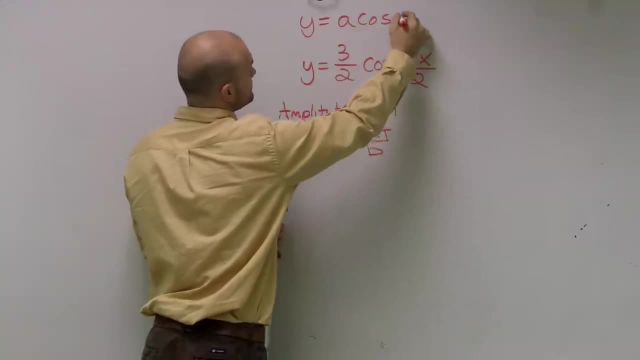 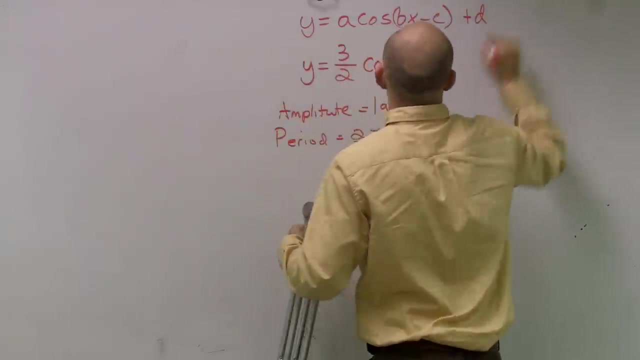 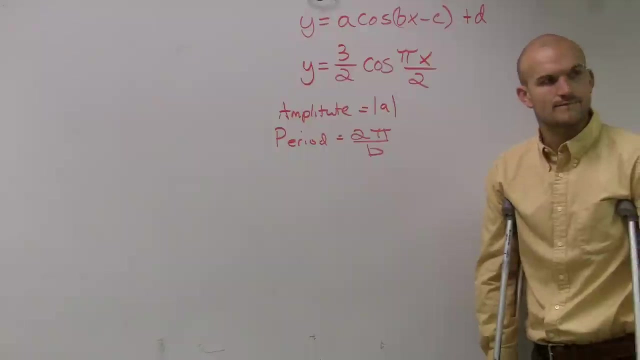 we have a cosine of bx minus c. Then we can say: plus d. Okay, Does that make sense to everybody? Yeah, Really Got it Okay. So now all I'm going to do is I need to determine what is my value, What is my number of b? 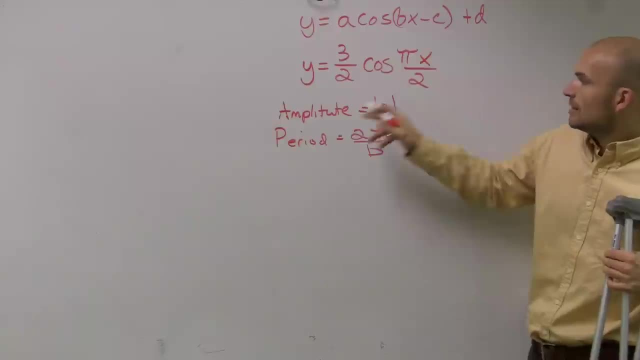 What is my number of b that is in front of my x? Well, actually, let's figure out a, So a. I look at what is the a. what's the number in front of cosine? Well, that's 3. 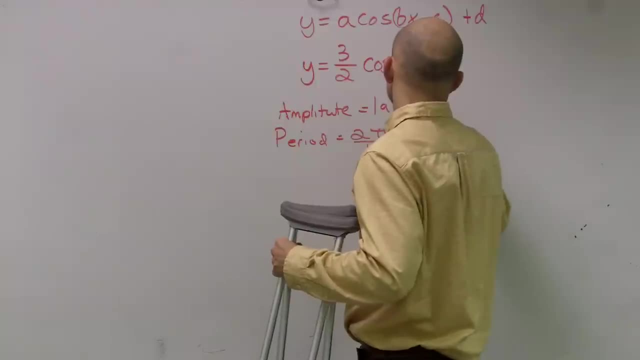 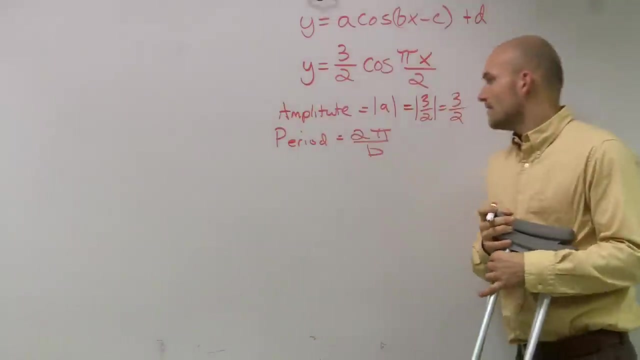 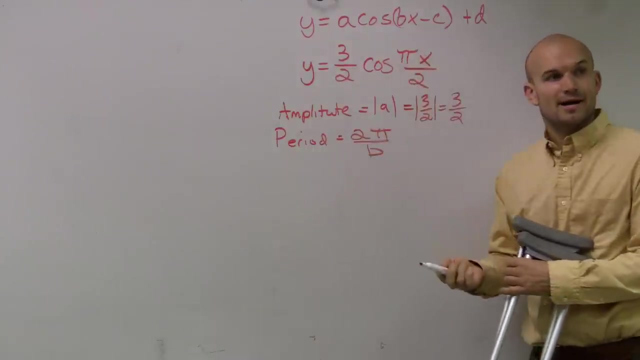 halves, right. So you can say the absolute value of positive 3 halves is obviously 3 halves, right. Then if I look at here, I say 2 times pi divided by b. So what is my number that's in front of b? Well, a lot of students will say it's going to be pi. But 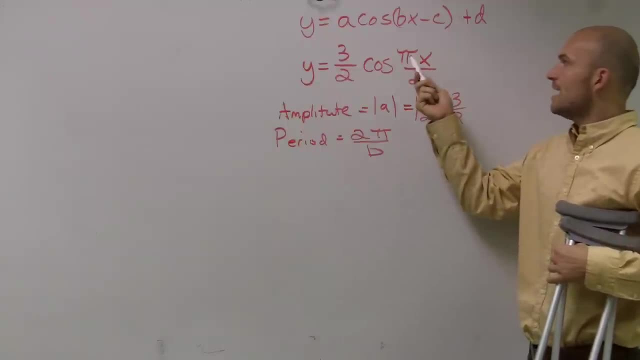 remember it's going to be pi. So what is my number that's in front of b? Well, a lot of students will say it's going to be pi. So if I look at a variable and I say: you know, free x, we know that x is being multiplied by 3, right. And then if I say divided by 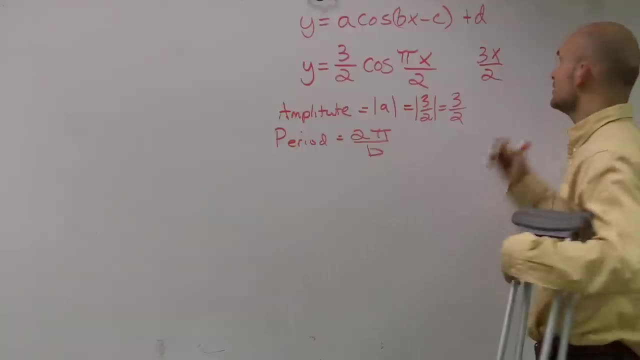 2, we know that my variable now is being divided by 2 as well. We can do that operation in the same aspect. when you multiply a fraction times 3 halves. It's the same thing. Multiply by 3, divide by 2. It's the same thing as multiplying by a fraction. So really, our